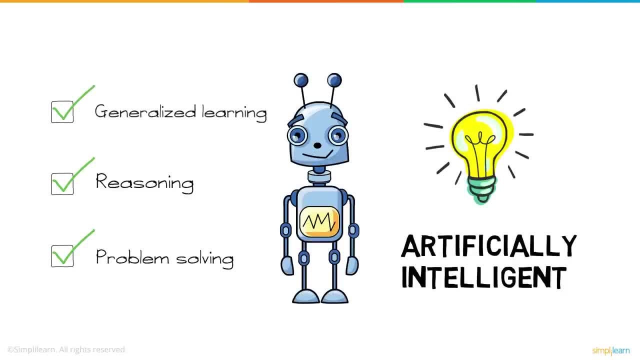 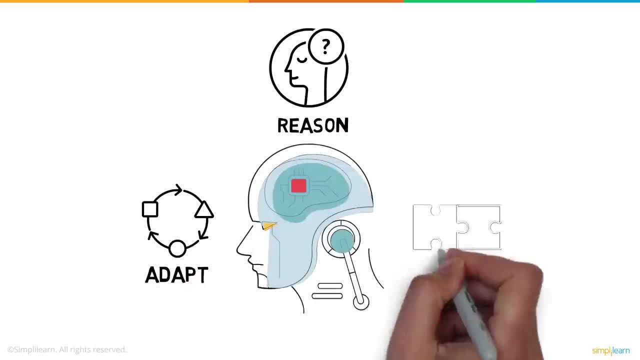 These three capabilities make the robot artificially intelligent. In short, AI provides machines with the capability to adapt, reason and provide results. The robot is now able to use the AI robot to solve problems, solve problems and solve solutions. Well, now that we know what AI is, let's have a look at the two broad categories an AI is classified into. 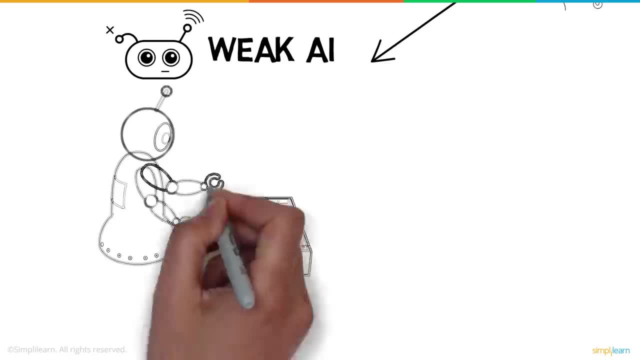 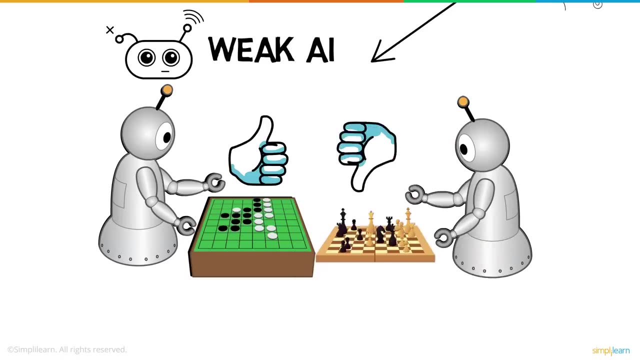 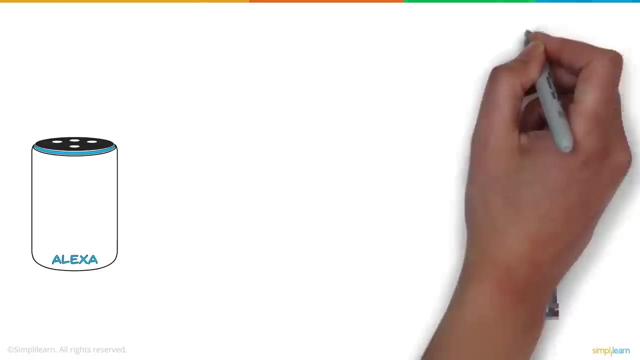 Weak AI, also called Narrow AI, focuses solely on one task. For example, AlphaGo is a maestro of the game Go, but you can't expect it to be even remotely good at chess. This makes AlphaGo a weak AI, Since it can perform multiple tasks. 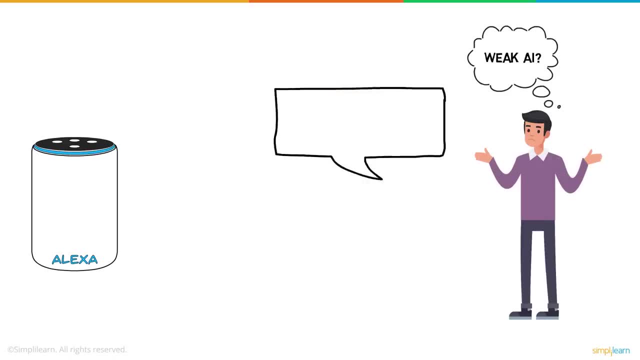 Well, that's not really true. When you ask Alexa to play Despacito, it picks up the key words Play and Despacito And runs a program it is trained to. Alexa cannot respond to a question it isn't trained to answer. 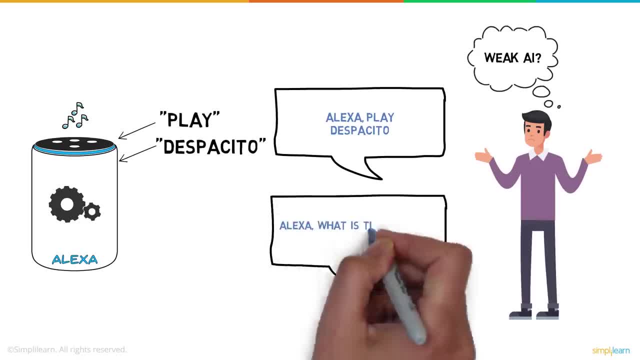 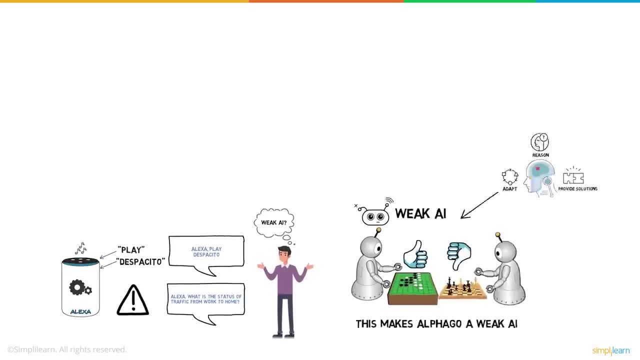 For instance, try asking Alexa the status of traffic from work to home. Alexa cannot provide you this information as she is not trained to. Alexa cannot provide you this information as she is not trained to. And that brings us to the final question. 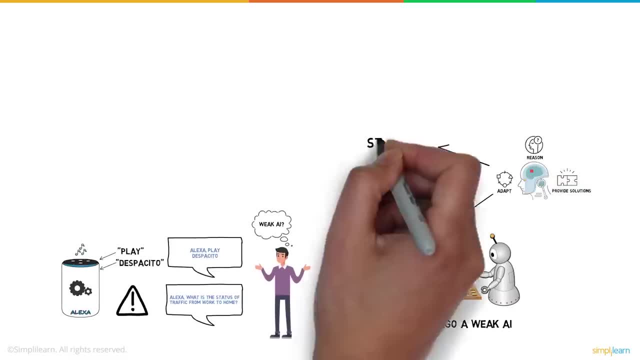 The final question is: why can't you connect to another network? And that brings us to the final question. And that brings us to the final question. And that brings us to the final question, brings us to our second category of AI: Strong AI. 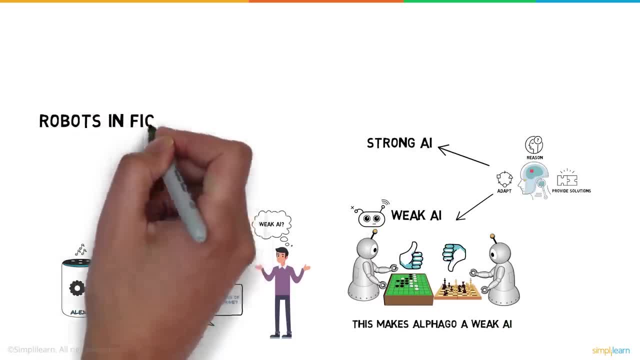 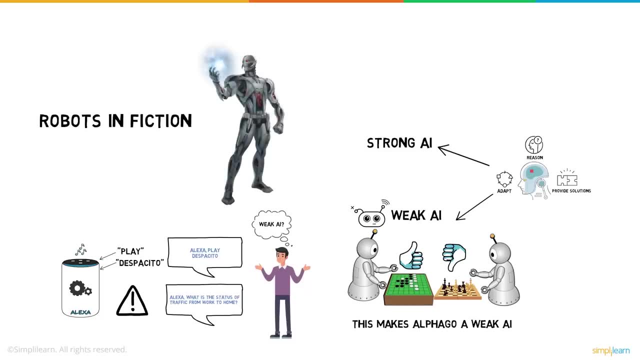 Now this is much like the robots that only exist in fiction as of now. Ultron from Avengers is an ideal example of a strong AI. That's because it's self-aware and eventually even develops emotions. This makes the AI's response unpredictable. 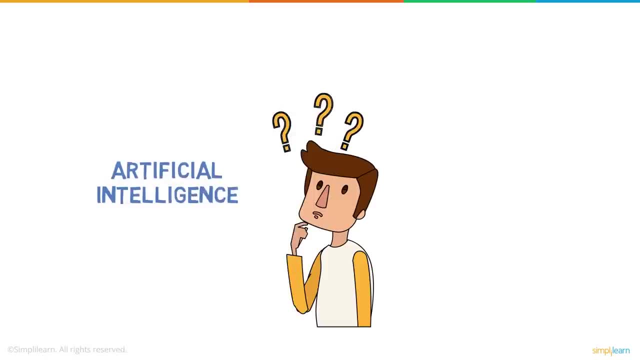 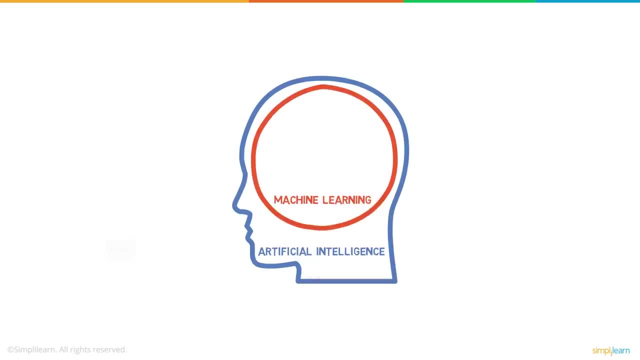 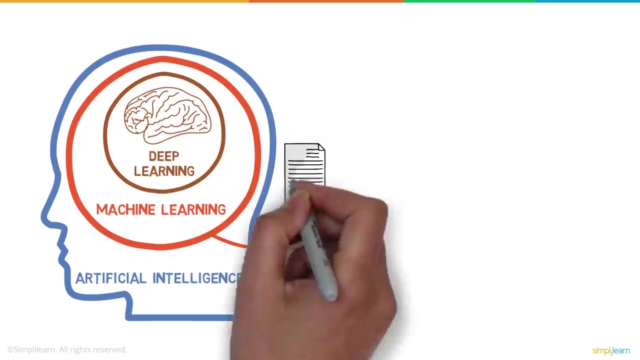 You must be wondering well, how is artificial intelligence different from machine learning and deep learning? We saw what AI is. Machine learning is a technique to achieve AI, and deep learning, in turn, is a subset of machine learning. Machine learning provides a machine with the capability to learn from data and experience. 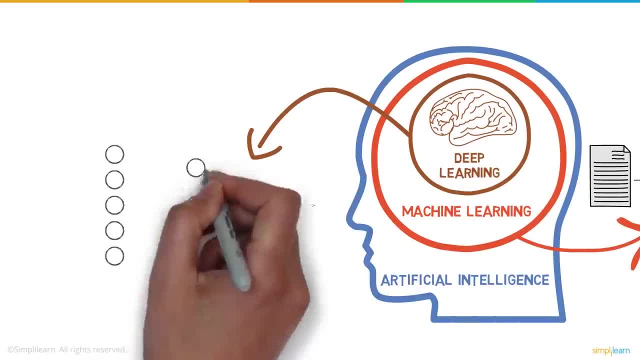 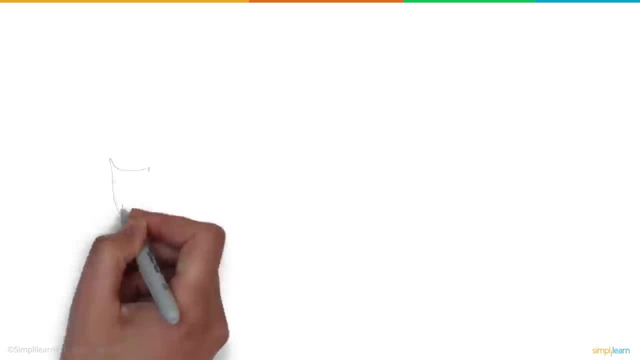 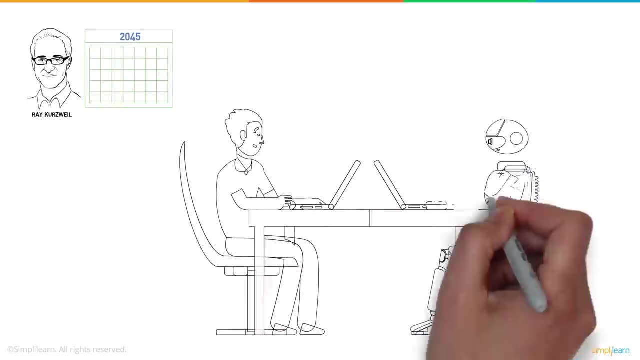 through algorithms. Deep learning does this learning through ways inspired by the human brain. This means through deep learning, data and patterns can be better perceived. Ray Kurzweil, a well-known futurist, predicts that by the year 2045, we would have robots as smart as humans.